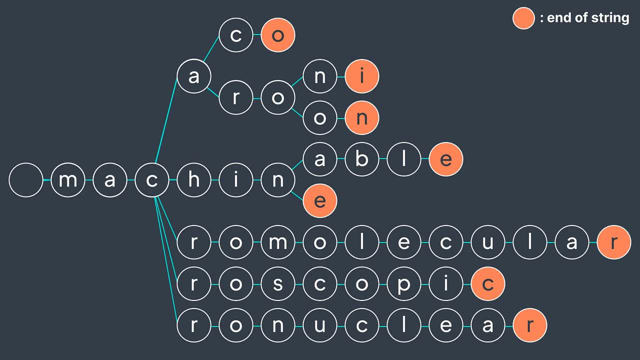 Heinable and Hein both start with hen- we store once. And romolecular, roscopic and roNuclear all start with ro, we store once. And we can't optimize anymore. What we did now is building the trie of these words. Each root to end of string node represents. 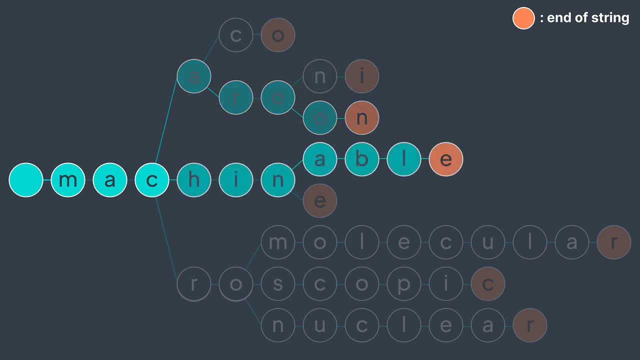 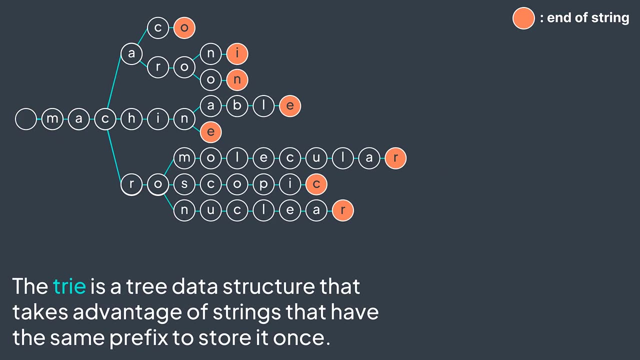 a string. We have macaco, macaroni, macrune, machinable machine, macromolecular, macroscoping and macronuclear. The trie is a tree data structure that takes advantage of strings that have the same prefix. 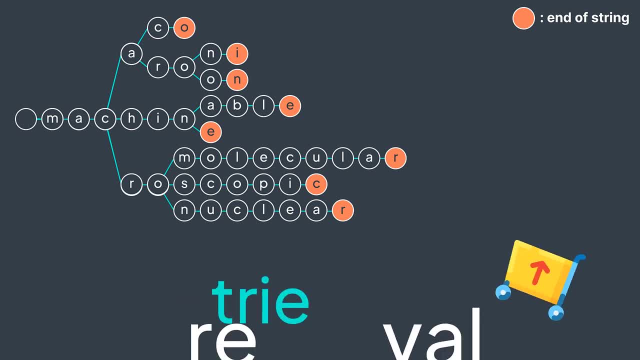 to store it. once The word trie comes from retrieval, It has an efficient retrieval. Instead of comparing the string we're searching for with all the strings, which is the case when they're stored in an array which can cost O, we just traverse the trie by moving to the next. 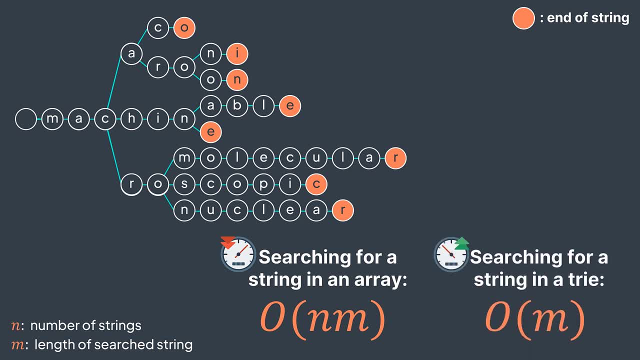 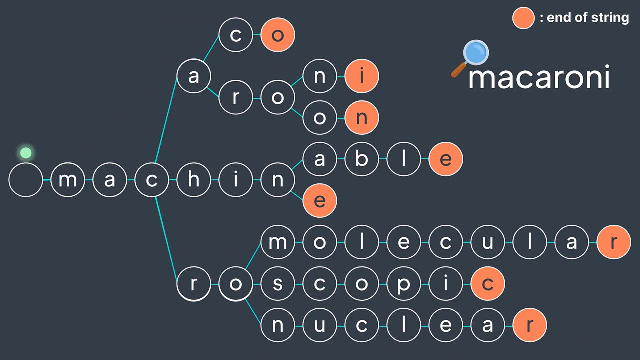 level at each iteration, which costs O only where m is the length of the string we're searching for. For example, if we search for macaroni in this trie, we start from the root and we go down in the tree. m, a, c, a, r, o, n, i And i is an end of word. so we found it without. 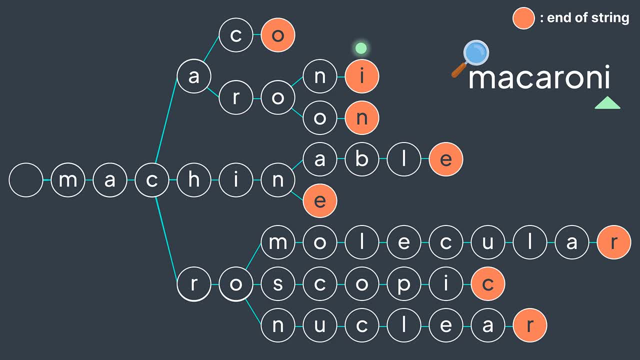 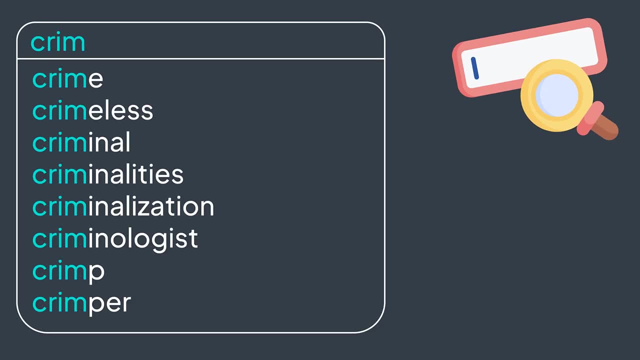 comparing it with all the words. Another advantage of the trie is that we can use it to implement the auto-complete feature, where you write something and it suggests you the words that start with what you wrote. It's good to implement it with the trie because, for example, if we want all the words, that's 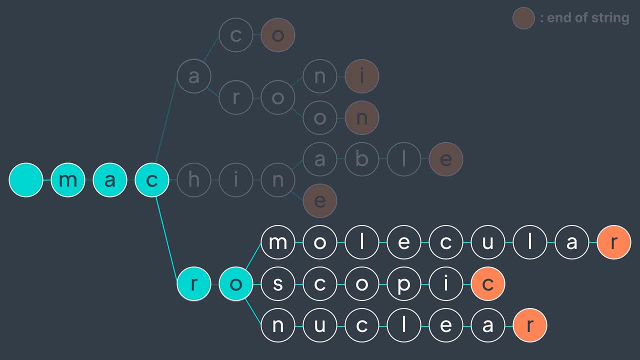 start with macro. we just traverse its characters in the trie and we find the sub-tree that contains all of them Here: macromolecular, macroscopic and macronuclear. I will show you how to implement the auto-complete feature in the next video. 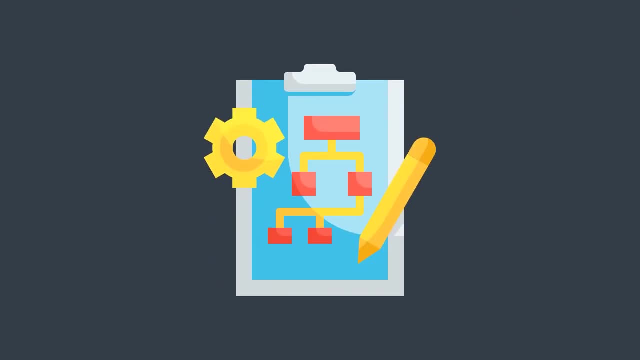 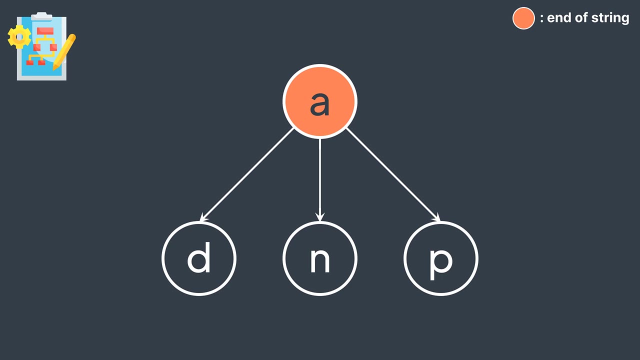 But now let's move to the trie implementation. In a trie node we want to have 3 information, The character, the references to children and a boolean that says if there is a word that ends in the actual node, Because words. 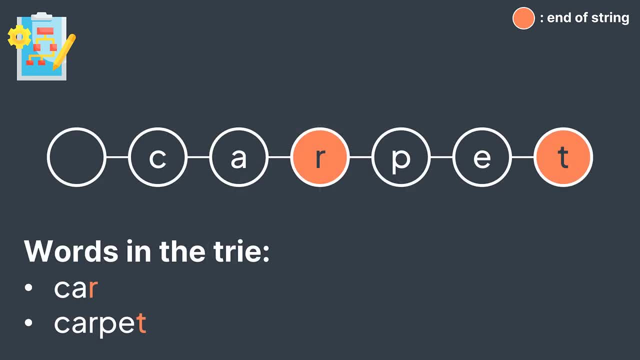 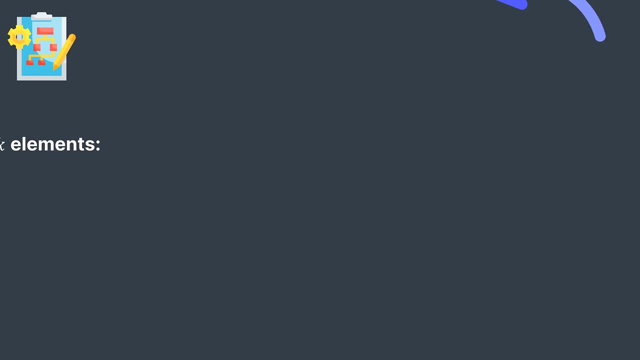 don't necessarily end in leaves. we have current carpet. we have to put the boolean in the node rtrue to say that we have the word car. Otherwise we would have the word carpet only in the try, And there exists multiple implementations for it. I'll show you four of them. The first one is to put an array of k. 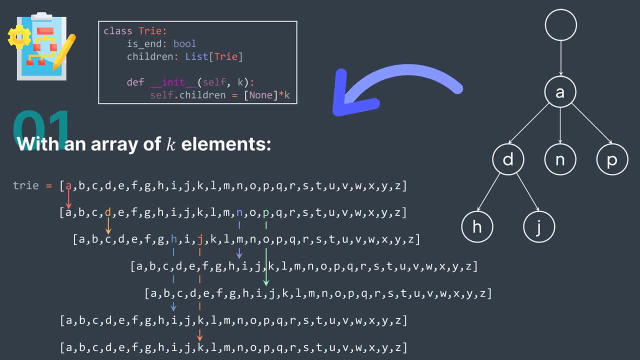 elements where k is the length of the alphabet. For example, if we're dealing with lowercase letters only, we put in an array of 26 elements, one for each letter. An element can either be null or contain a reference to a node, depending on if we have a string that passes from that. 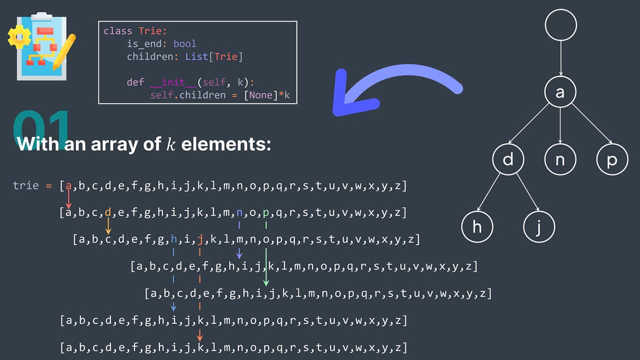 letter. I know that the left figure is a little bit confusing, but I've called the elements that are not null. and where do they point? In reality, letters are not stored. we work with indices only. For example, the first array represents the root. it has only one children. the letter A. 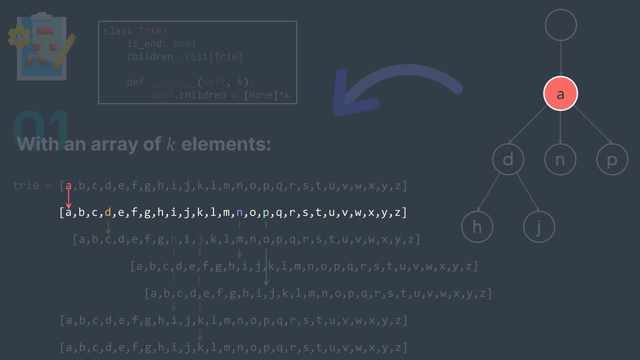 Then the letter A has three children: D, N and P. each one of them is pointing to a node. N has no children, P has no children, N has no children and D has two children, H and G. Each one of them points to a node. 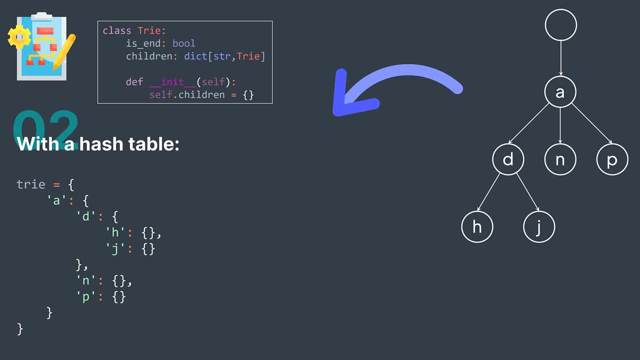 The second possible implementation is to use a hash table that maps characters to nodes. The key is a character and the value is the node that it points to. Third possible implementation is to use an array of children of type node. And the fourth possible implementation is to save the reference to the first children only. 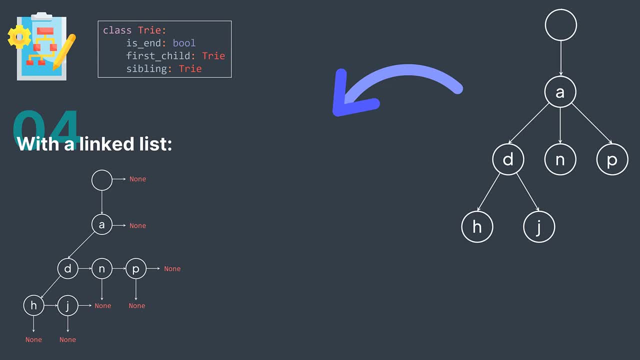 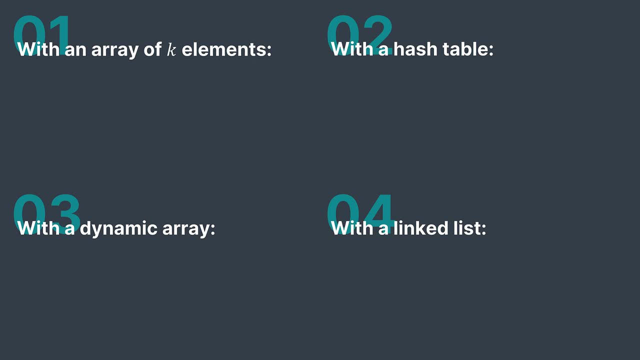 but to also save the reference to the sibling. So children will look like a linked list. The third possible implementation is to use a hash table that maps characters to nodes. But which one to choose? The answer is: it depends. It depends on your priority. 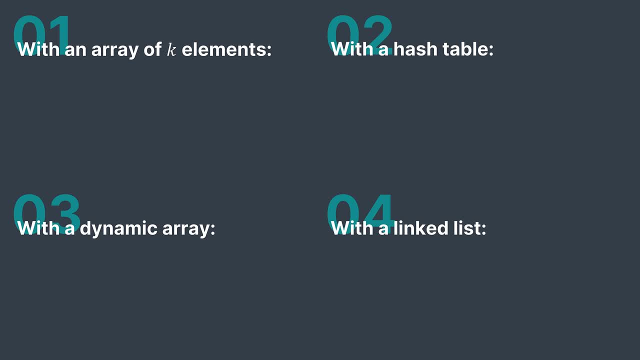 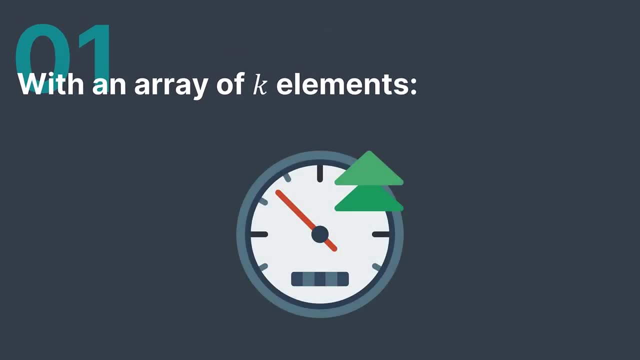 either time or space efficiency, the size of the alphabet, the density of children, etc. Some of them are more time efficient and some of them are more space efficient. For example, the first one is pretty fast: Accessing a node is O, because we're using an. 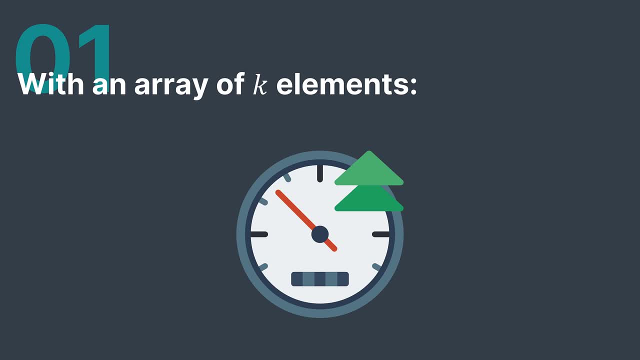 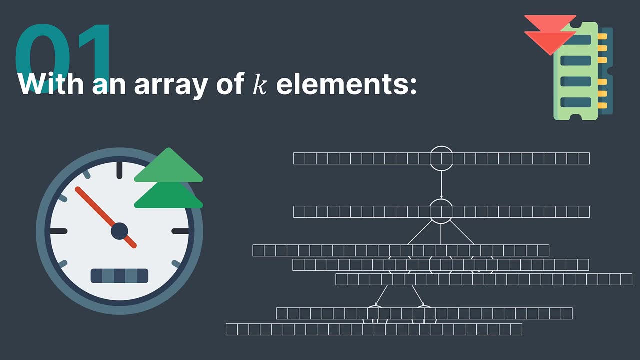 array and we can directly get the index of the character we search for. But the problem is that for each node we store k elements, where k is the size of the alphabet. So if we have a large alphabet and or we don't use a lot of different characters, 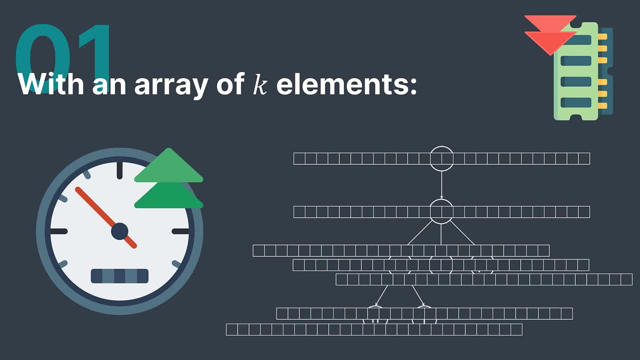 there would be a lot of waste of space, And don't think that, nah, it's fine. we have a lot of space nowadays because the space inefficiency has a huge impact when there are millions of nodes. The last implementation is quite the opposite: it doesn't waste much space because we deal with. 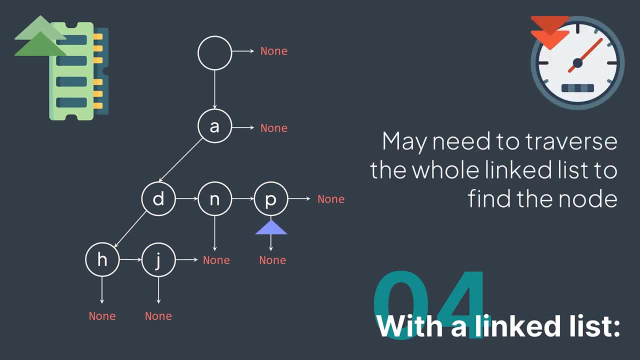 links only, But we may need to traverse the whole sibling's linked list to find the one we're searching for, which can be a waste of time. This is why we can try to limit this by putting a string in the left of the left of the left For this video. we will work with the second. 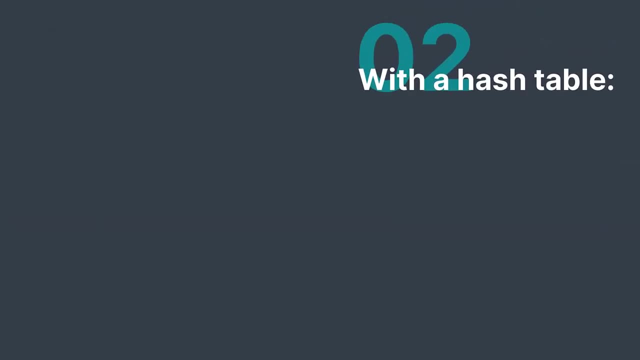 implementation, the one that uses a hash table, And we can even avoid to store the node's character because it's already done in the hash table key. So our try node will contain two attributes. a boolean is n, that says if there is a string that ends in the actual node. 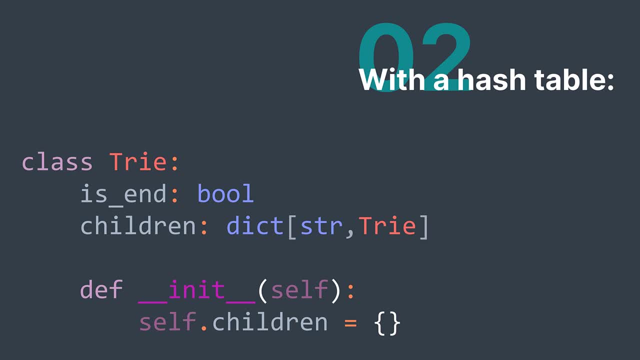 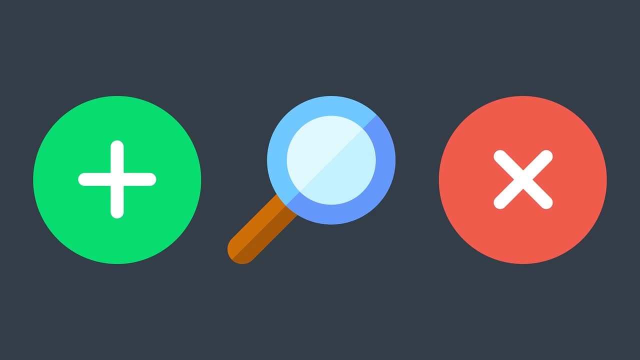 and a hash table, children, where we map characters to nodes. Now we need to know how to insert, search and delete a string and how to retrieve all strings of a try. Let's start with insertion. For that we need the root of the try and the string that we're. 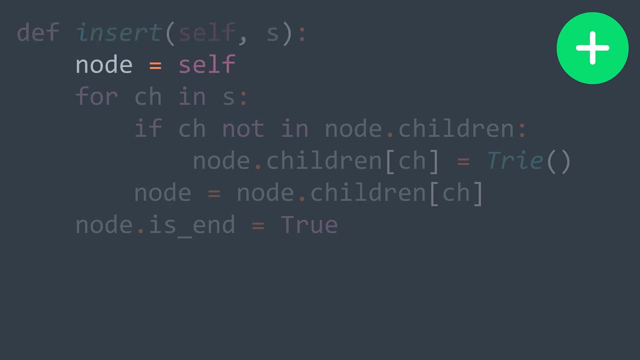 gonna insert, We create a node that is on the root. then for each character in the string, we move node to the node of that character if it's in children, And if it doesn't exist, we create it before doing so. After the loop, we set its end of the actual node to true. 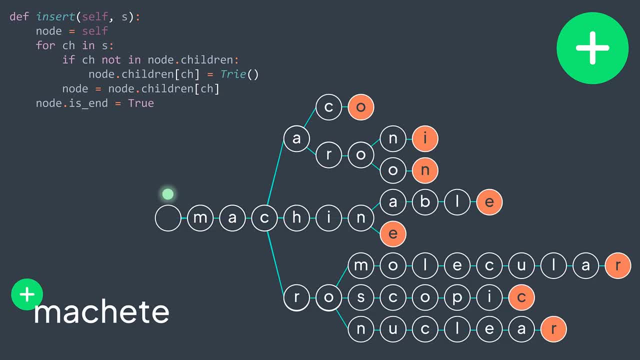 For example, we have this try and we want to insert the string machety. We start from the root. do we have m- Yes, we go to it From here. do we have a- Yes, we go to it. Do we have c: Yes. Do we have h- Yes. Do we have e: No, So we create it. 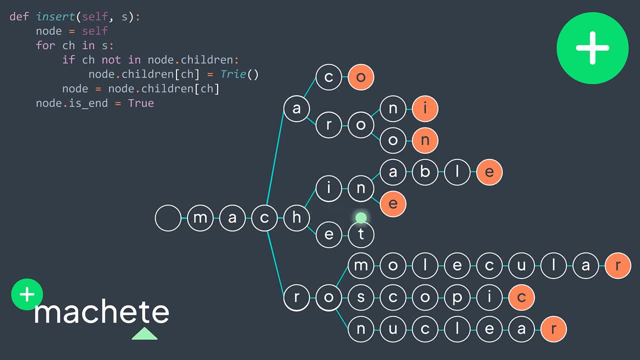 then we go to it. Do we have t? No, we create it and we go to it. Do we have e? No, we create it and we go to it. We finish traversing, so we put its end of the actual node to true. 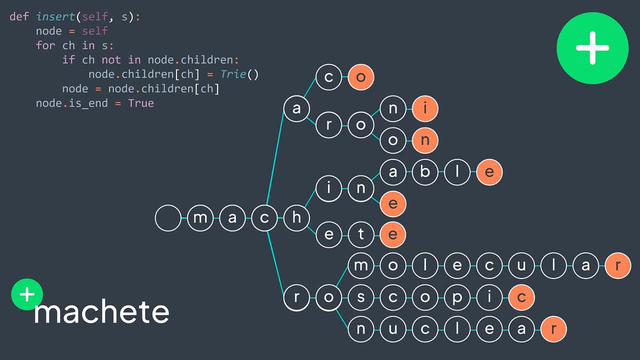 to say that we have the word machety. Let's insert another string, For example math m. we have the node Next character a. we have the node Next character t. we don't have, so we create it before we go to it. 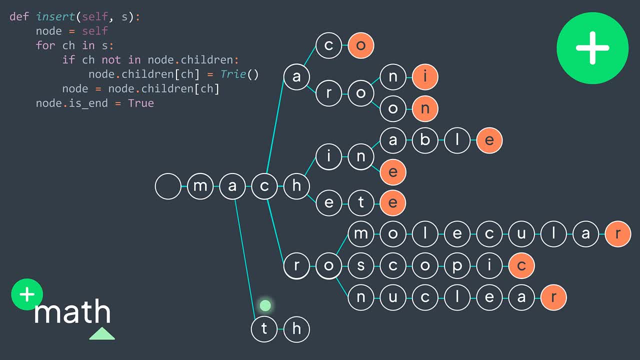 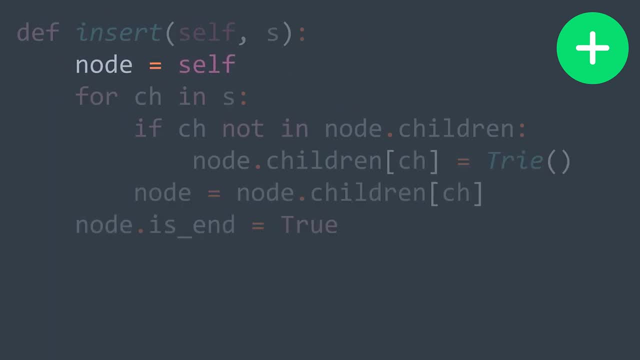 And last character h. same thing. We create and we go, We finish traversing. we put its end to true, By the way, in code, when we create a node and we assign to it self the equivalent of this. 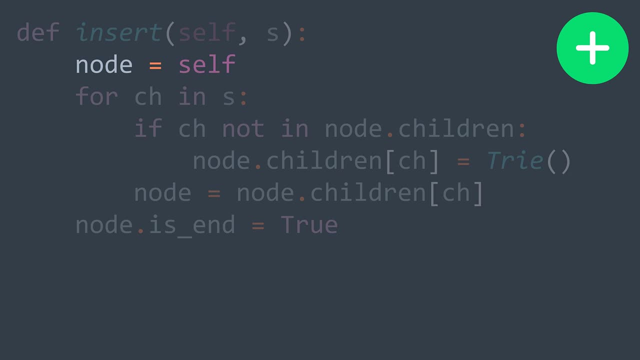 in some other languages. what we did is to create a node that starts on the root Self, represents the object itself. This method has an over-end time complexity, where m is the length of the string that we want to insert. Next operation: searching: We want to return. 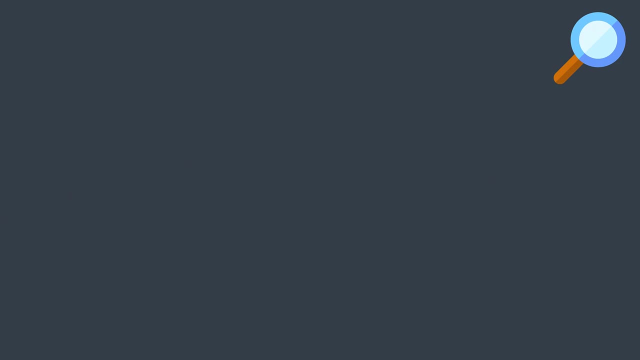 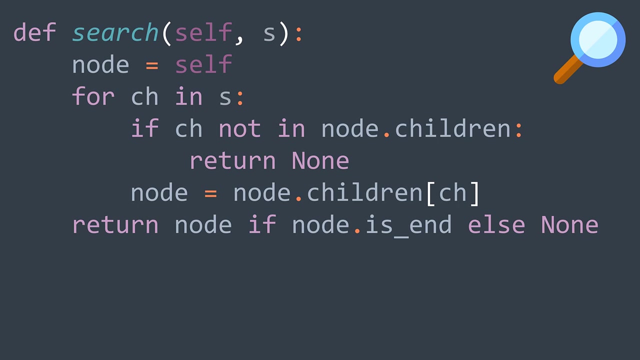 the node where the string that we're searching for ends For searching, we use the same logic as for inserting. It's just that when we don't find the node in children, we don't create it. it just means that the string doesn't exist in the trite, so we return null. 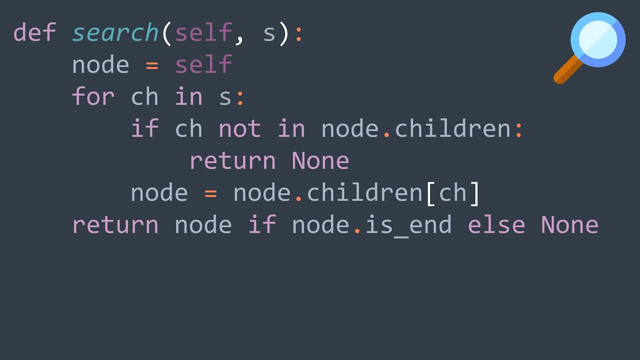 Else. we just set node to nodechildren of ch and we continue. After the loop we return the actual node. if it's an end of string, It represents the node where the string as ends, But if it's not an end of string, we return null. because even if we've 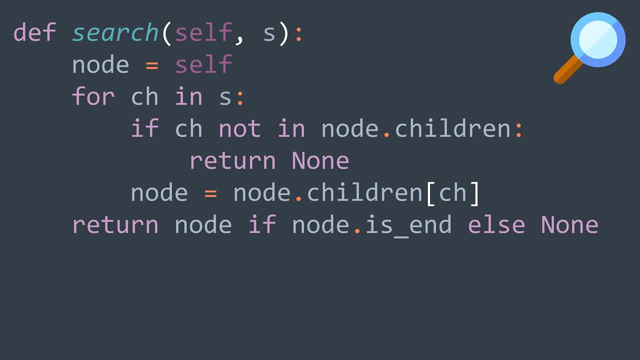 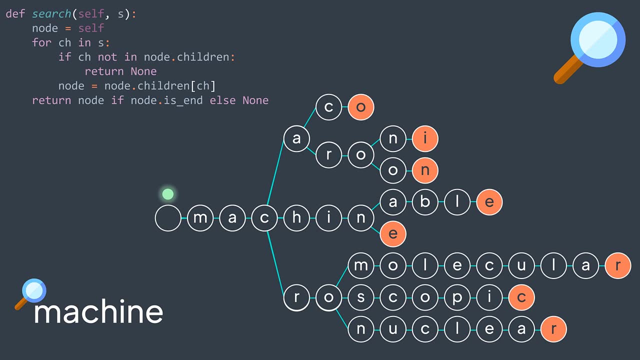 been able to find all the characters. but the last node is not an end of string, so the string doesn't exist in the trite. For example, in this trite, if we search for the string machine, we start from the root and we have m, a, c, h, i and e and we return this node. 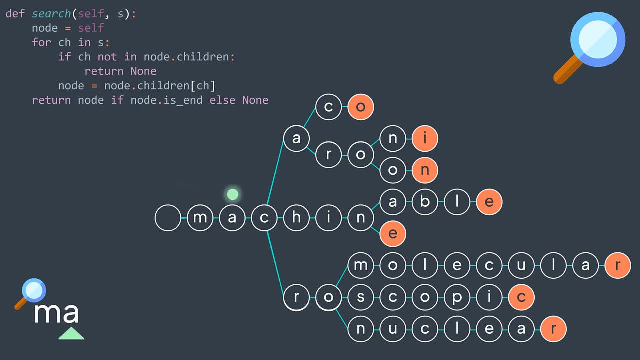 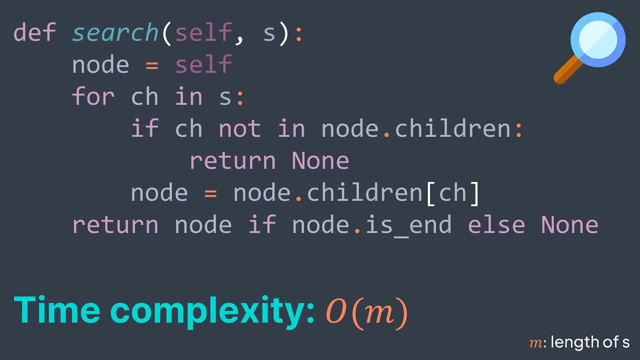 But if we search for the string m, a, we have m, we have a, but a is not an end of string. we return null. This method also has an over-end time complexity. Now for deleting a string from the trite. it's a little bit more difficult, because deleting a string shouldn't affect. 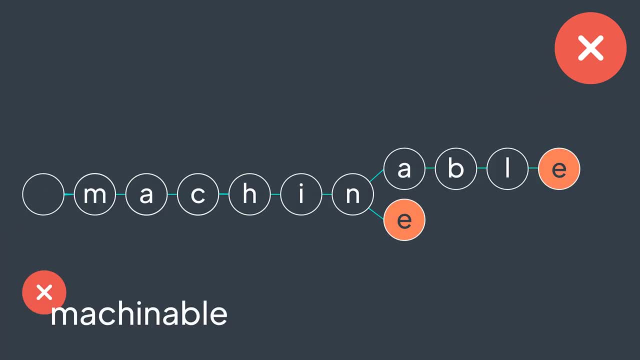 all the strings in the trite. Yes, we can just search for the last node of the string and set its end to false. it's not wrong, but we would have unnecessary nodes which cost space uselessly, So it's better to delete them, while being careful. 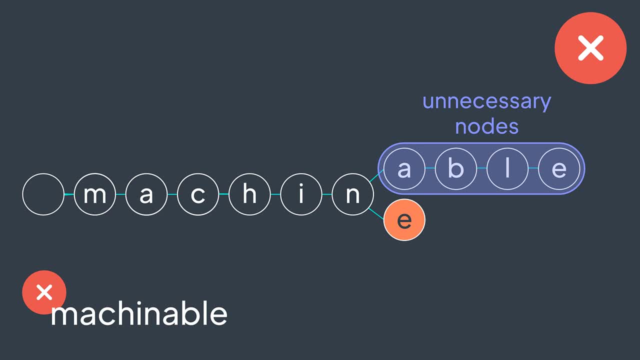 Let me give you some examples where we have to be careful. We have a trite that contains the words car and carpet and we want to delete carpet. If we just delete the nodes without being careful, we would also delete the word car, which is not intended. Another special case is when one of the 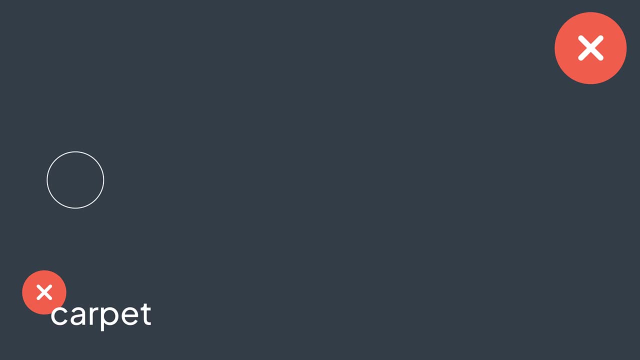 nodes that we want to delete contains all the children. For example, we have a trite that contains carpet and carry and we want to delete carpet. We delete the t, we delete the e, we delete the p, but we cannot delete the r because it has children. so if we delete it, we would. 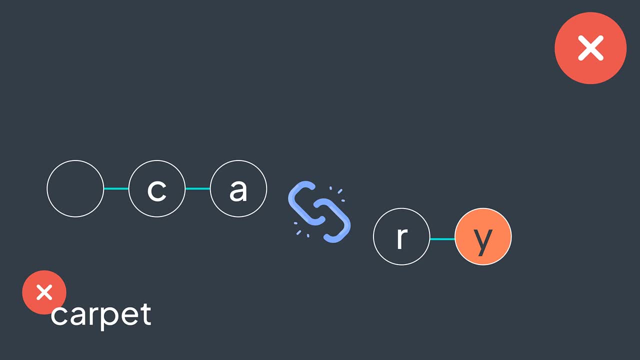 also delete other strings carrying our case. Third and last special case is when the last node of the string has children. For example, we have book and book and bookmark and we want to delete book When we reach the last node, which is k. 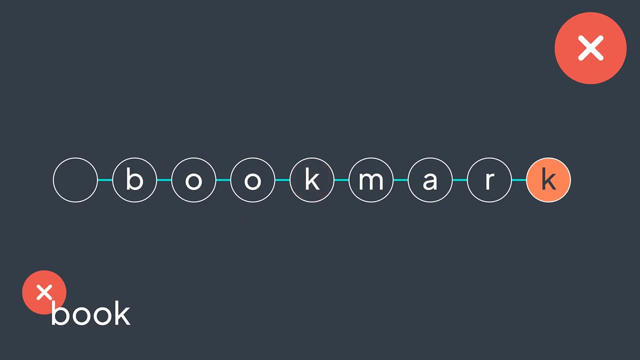 we set its end to false because it's not an end of string anymore, but we do nothing else. we can't delete any node. We would lose the string bookmark. otherwise. Ok, but how to implement deletion operation by taking into consideration all these special cases? 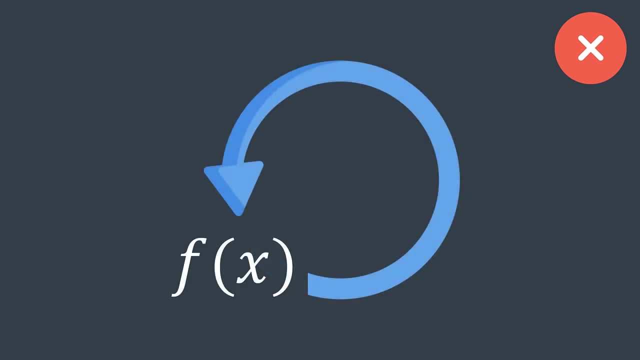 An interesting way to do so is by doing it recursively. Why? Because we want to reach the bottom of the string in the trite, which is the end node. then we go back to delete nodes that need to be deleted, And to do so recursively, we put the instructions after the recursive call. 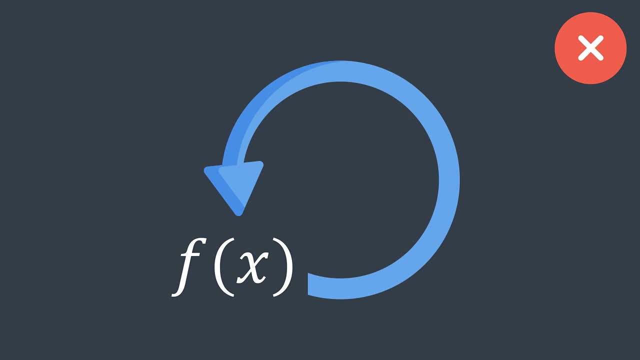 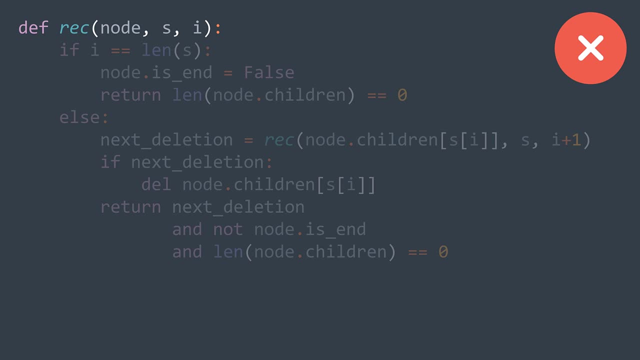 to start processing from the bottom and not from the top. We said that we need to stop deleting at some point, so our recursive function will be a boolean function. it returns if, yes or no, we continue deleting. The base case is when we reach the last node, we set its end to false and we continue deleting. 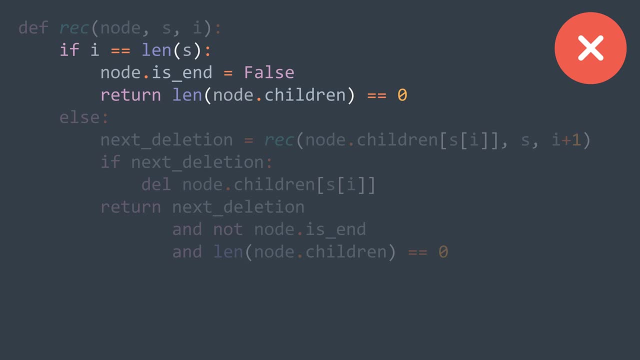 depending on if the last node has children or not. so we return numberOfChildren equal to 0. And in the recursive case we recursively call the function with the next node in the path of that string in the trite. this is why node becomes a children, whose character is s of i. 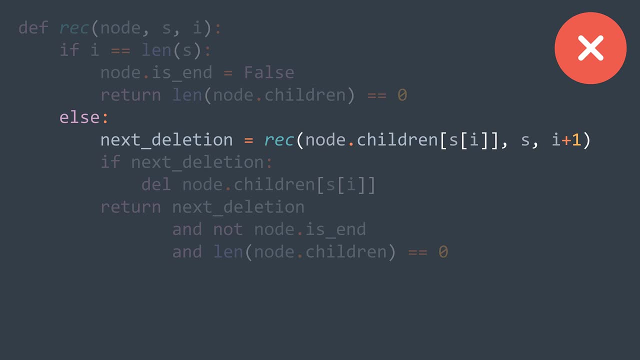 the actual character and i becomes i plus one to move to the next character After getting the result. if it's true, then we delete. We delete the children. that contains the actual character s of i. Then we have 3 conditions to continue deleting The recursive. 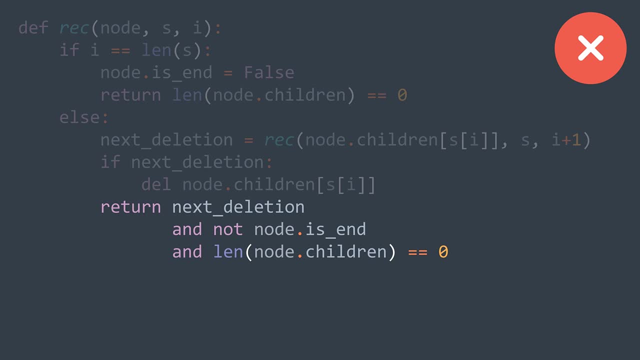 function return: true, the actual node is not an end of string. remember the con carpet example. and the actual node has no children. remember the carpet and career example. If all these conditions are respected, then we delete the actual node. so the boolean. 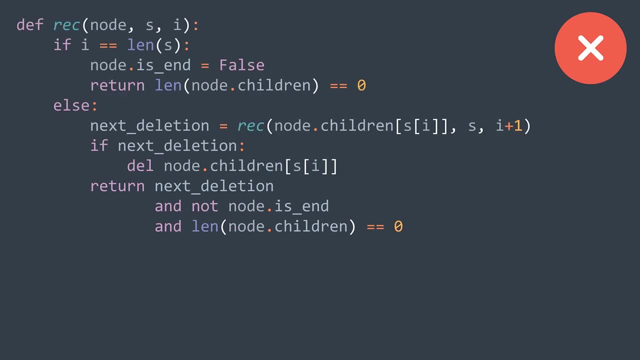 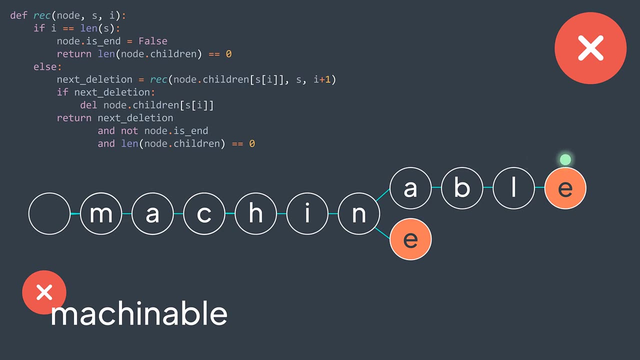 expression returns true. Quick example: we have this trite and we want to delete machinable which offers the nodes recursively m, a, c, h, i, n, a, b, l and e. Now base case: we set its end to false and we return true because the last has no children. 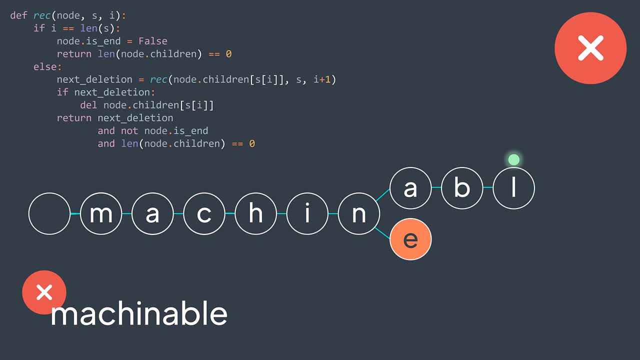 Back to this node. the call didn't return false, so we delete the child. and it's not an end of string and it has no children, so we return true. Same thing for this one. same thing for this one and for this one. 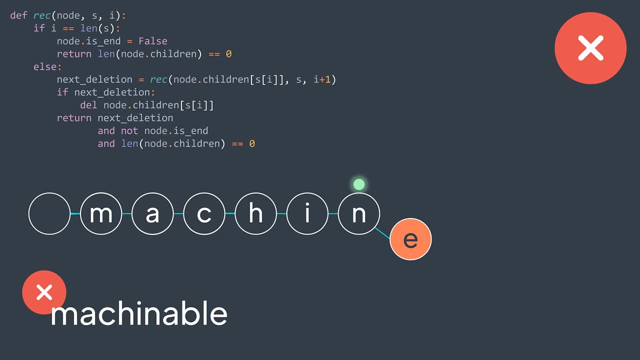 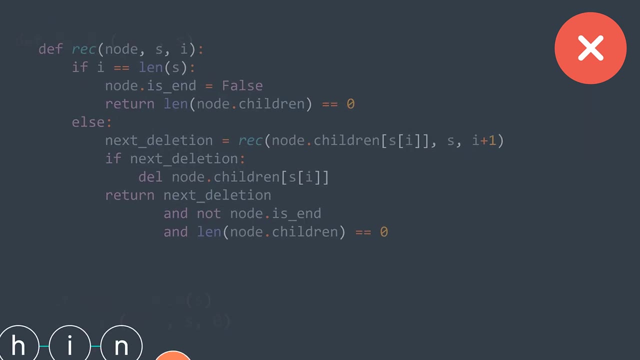 the function returned true, so we delete the child, But the actual node still has children. we return false And now all remaining calls don't delete and return false. And we deleted the string machinable without affecting all the strings, And in the non recursive function we first make sure that the string that we want to delete exists. 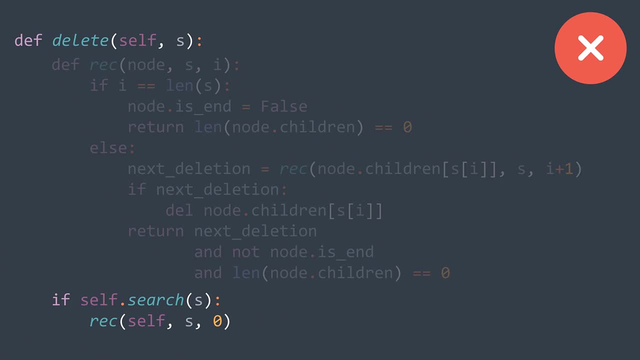 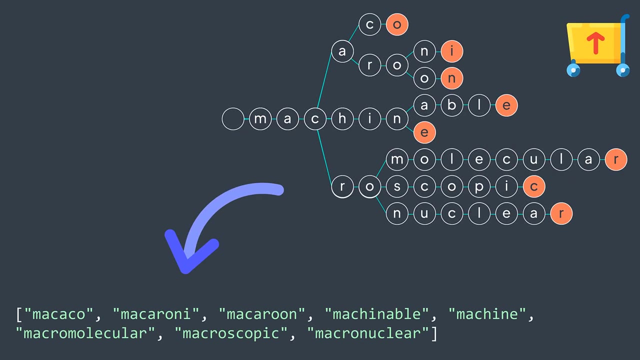 only when the search function returns a positive result. This method also has an O complexity. Last manipulation: retrieving all the strings of a trie. This one will be useful for the autocomplete feature that we will see in the next video. Retrieving all the strings is equivalent to finding all the route to end of string node. 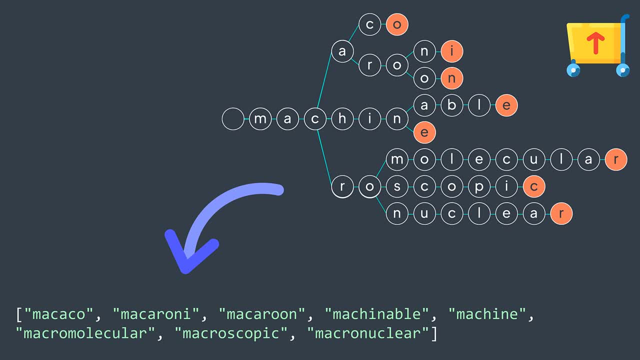 paths, because each one of them represents a string. What we're gonna do is to traverse the trie in depth first, while adding the actual string to the array of strings. every time we find an end of string node. So the function needs three parameters: the actual node, the string. 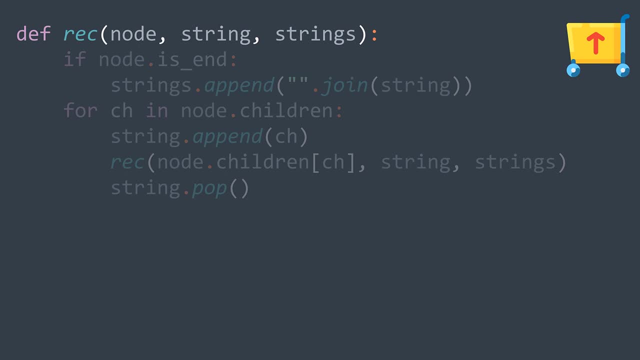 we're building and the array of strings. If the actual node is an end of string node, we join the characters and append the string to the array of strings. After the condition for each children character ch, we append the character to the string we're. 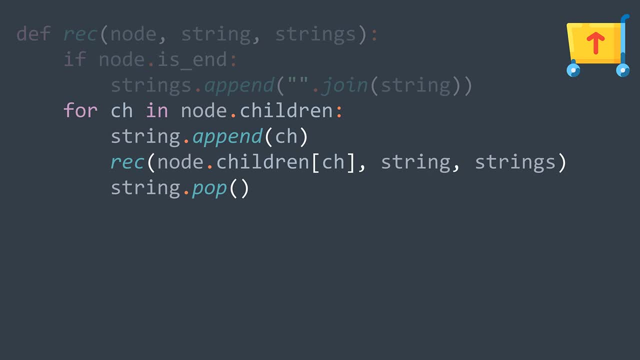 building. we call the recursive function, starting from the children node and we remove it after it. It's the technique we learned in the path related tree problems, video Recursive function And in the non-recursive function we create the array of strings. we call the recursive function. 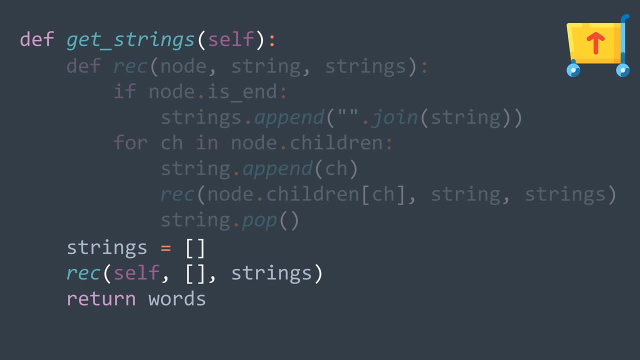 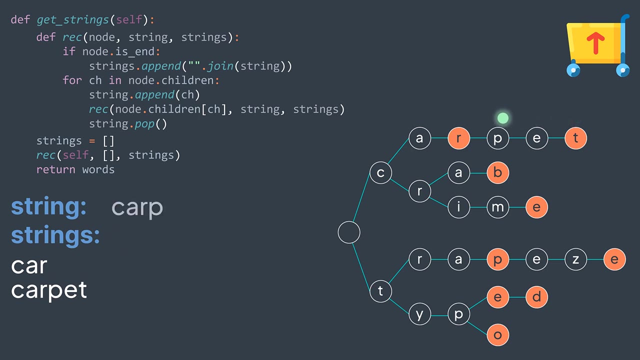 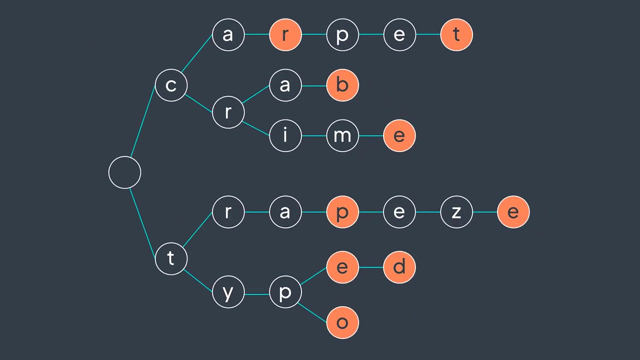 to fill it and we return it To better understand. this is what happens with this example. We'll go into more detail in the next video. We've reached the end of this video. In this one we talked about the trie data structure. 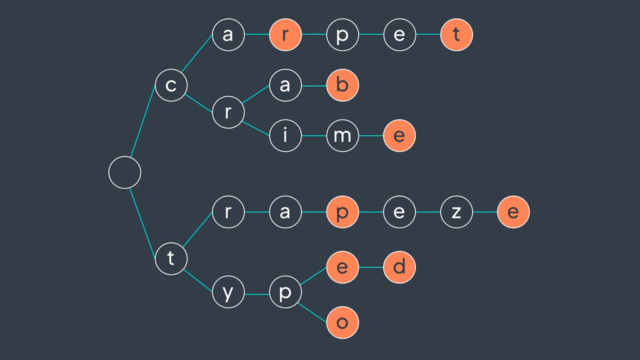 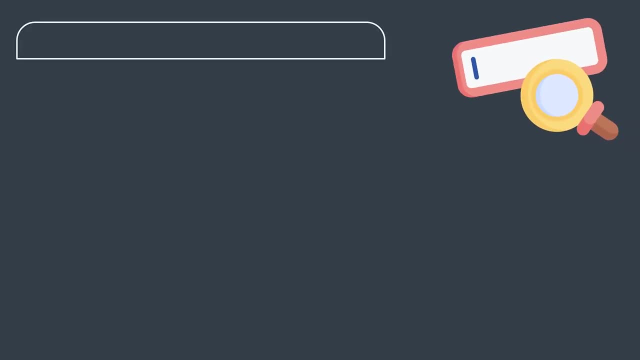 In interesting data structures to know. we talked about its advantages, some different implementations and implemented its main operations. In the next one, we'll use it to implement the autocomplete feature, So make sure to subscribe to the channel. I hope that I've been able to explain to you the trie data structure process and I hope that you. 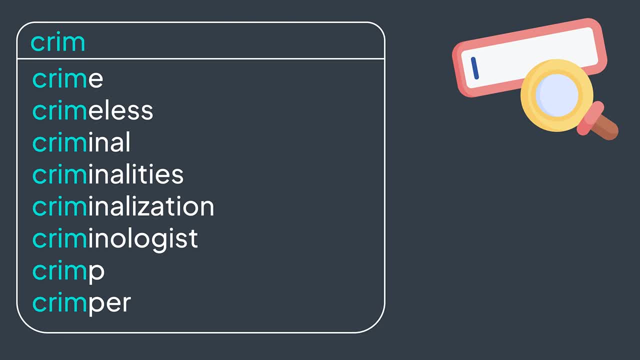 enjoyed it and I'll see you in the next video. I hope that I've been able to explain to you the try data structure. tell me in comments if it's the case and see you in the next one.